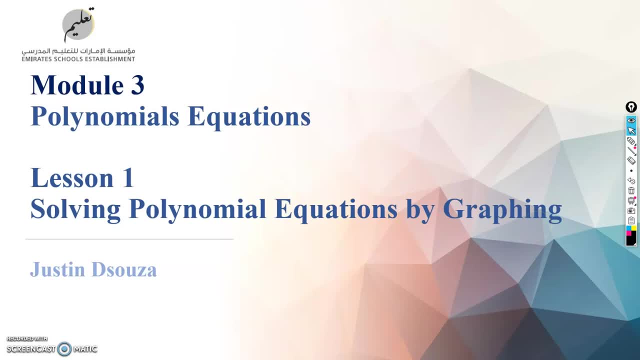 lesson I want to quickly tell you: please do subscribe to my channel. It would really mean a lot, and I want to thank all the subscribers- so many hundreds of subscribers. I thank you so much. I greatly appreciate it and please do share this this. 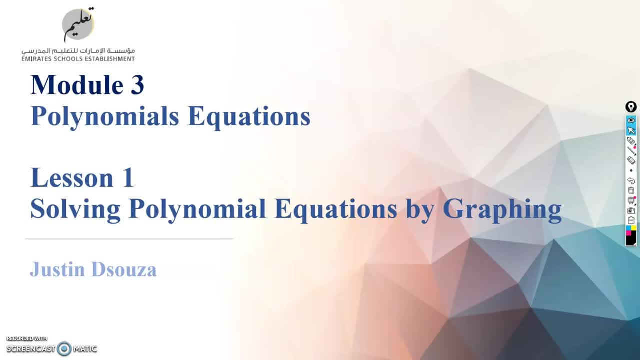 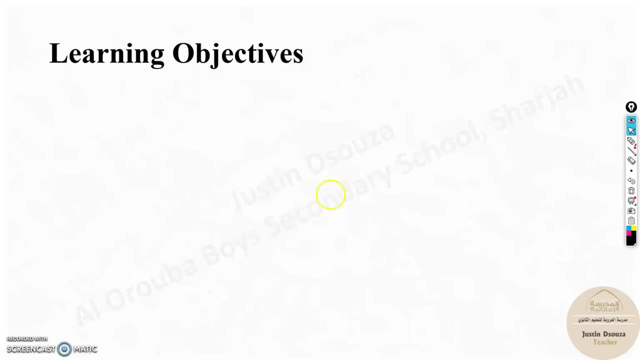 video with your friends. You can share the links with your friends, who might find it useful as well. Now moving on to the lesson. this is a short lesson, you know. so only one learning object here in this, that is, to solve polynomial equations by graphing. Before we start this, 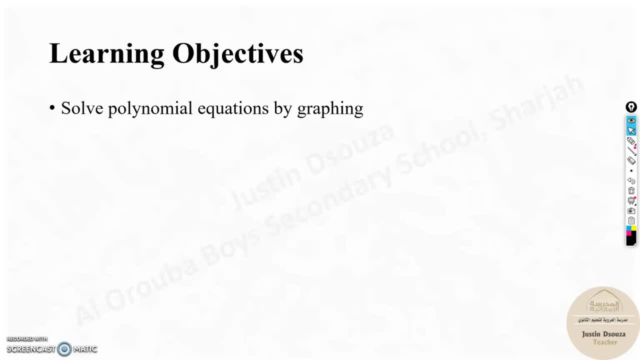 lesson you might have remembered, the last module was also on polynomials. Yes, but this is on polynomial equations. We will solve them. We will find the solutions for the equations. So that is what we are going to do. So let's get started. 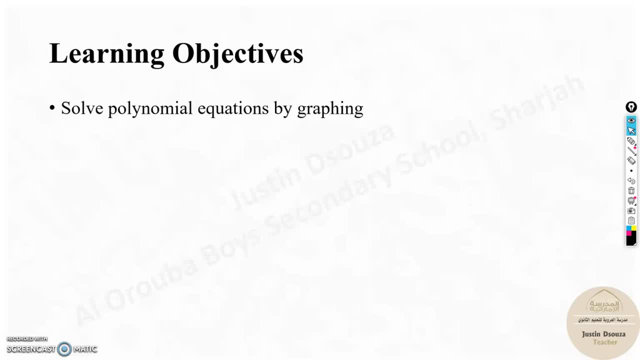 In the last we did operations on polynomials: Adding, subtracting, multiplying, binomial, polynomial, dividing- But here it is about polynomial equations. Now it is about graphing The keywords. are it's only one keyword? sorry, the keywords is polynomial equations. 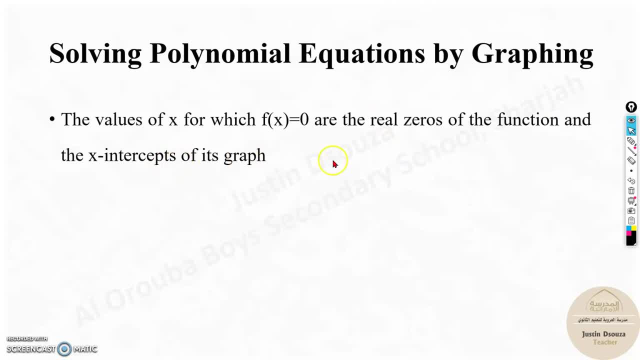 Now solving polynomial equations by graphing. Now, over here, let me show you this. This is a polynomial. Now, whenever there is equal to equation comes. Equation means you're equating something with other thing, So this is a polynomial equation. 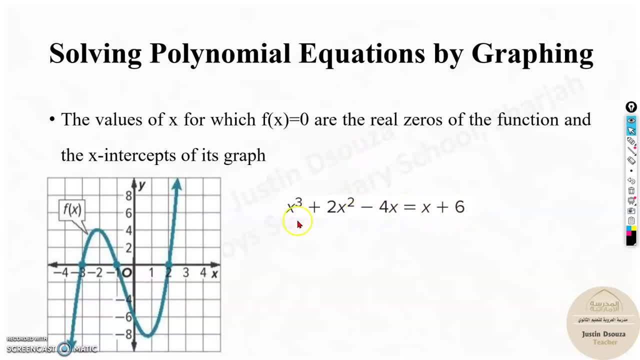 Why? Because this is equal to. How do you solve this? If you want to solve, that means it is the intercept, the x-intercept values. That is the solution for the polynomial equation. That x-intercept is also called as the solutions. 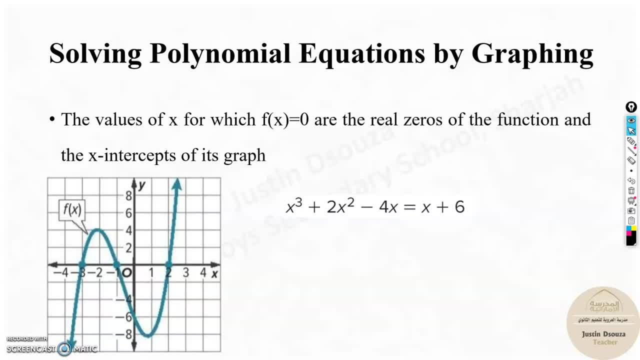 Now, how would you solve it? Now, if you recall before, you might have studied. if I want to know the x-intercept- okay, this one- I should just make the function equal to 0.. If this is the function of the graph, make it equal to 0.. 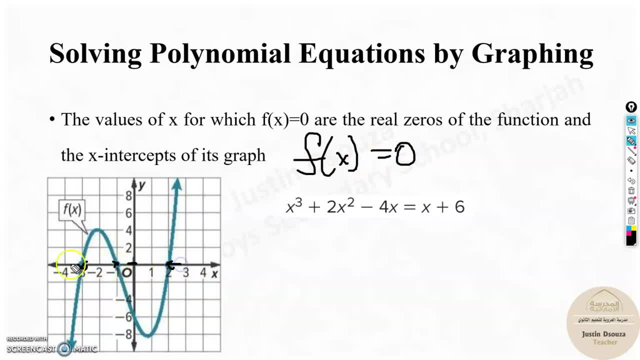 Why. That means where is y equals to 0? At the x-intercept values. So what you need to do is you need to rearrange this and get everything to one side. Now, since this is higher power, let's take everything to the other side. 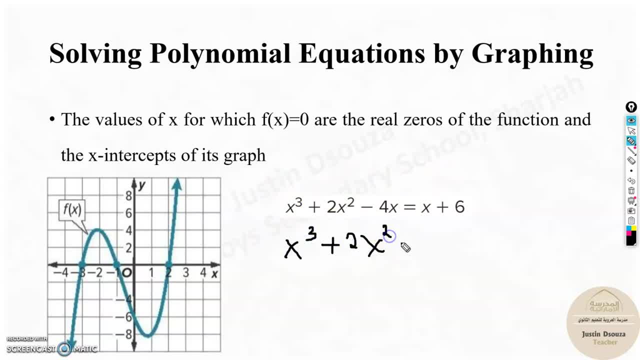 x to the power. So this is going to be minus 4x plus 2x, squared minus 4x and this becomes minus x. or subtract both the sides by minus x, It will be totally minus 5x and this will be negative 6.. 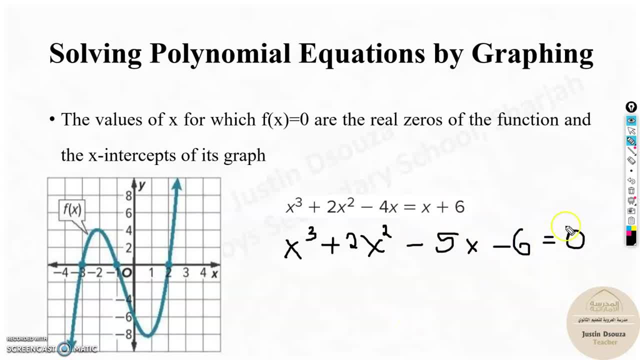 That is basically equal to 0.. Now that is basically the function f of x. So now you need to make the function equal to 0 and then solve. you will get the answer So you can see over here they have rearranged it. and then you make this equal to 0 and solve. 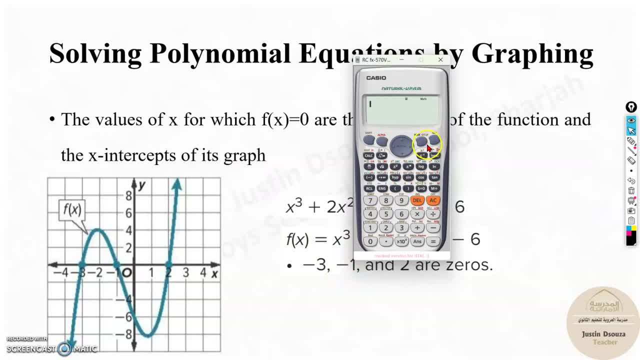 These are the zeros. How would you solve them? It is by pressing mode phi and over here up till cubic you can solve by pressing 3.. The coefficients are. you can see the coefficient before x cubed is 1.. 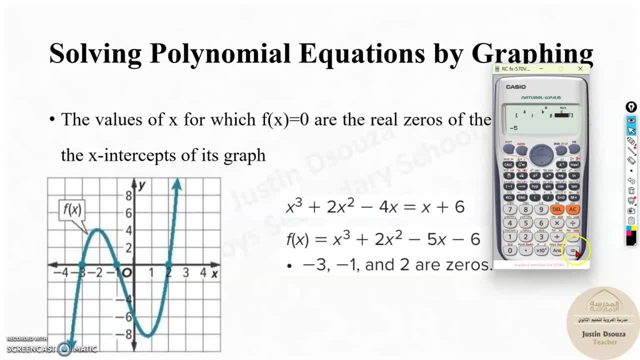 Then it's 2 before x, squared minus 5.. And lastly, we have minus 6.. And the answer are: sorry, did I do anything wrong? It's 1, 2, minus 5.. Sorry, it's not minus 6.. 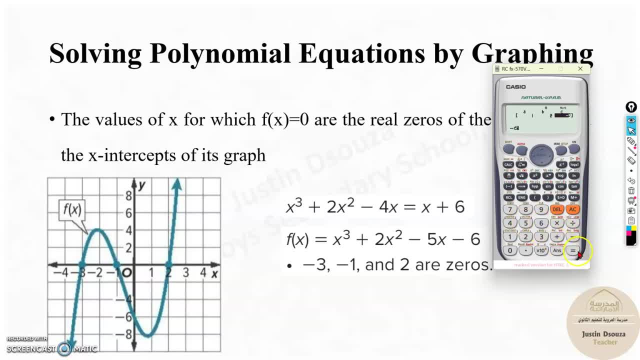 It's minus 5 and minus 6.. Now we will get the correct answer. Okay, I have done a mistake that I have just I pressed mode phi and 3.. It is mode phi and 4.. You can see, the cubic is 4.. 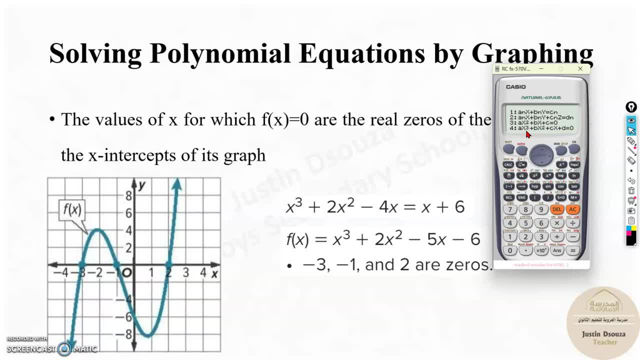 Now, it's good that I made this mistake. I'm not going to cut this part, I let it be The reason being. now, in your exam, you must be very careful on which, on which, equation you select If it's 4.. 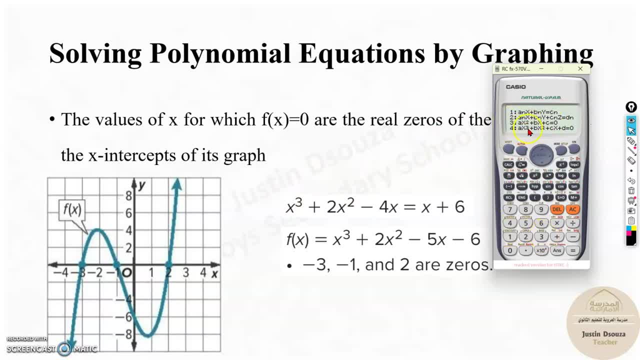 If it's quadratic, it's 2.. It's option number 3 over here. Since it's cubic power 3, select 4.. And now press the coefficients 1,, 2,, negative 5. And lastly, we have negative 6.. 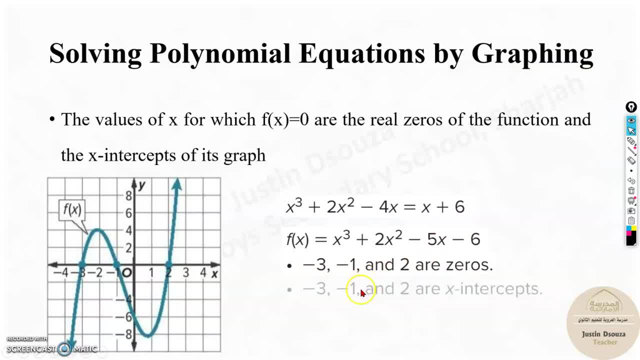 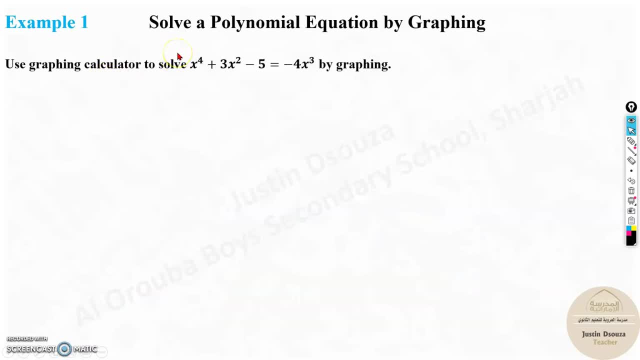 I hope this is clear. It is 2, negative 1, and minus 3.. So these are the answers. They are the zeros or the eccentricities. Now we will solve a problem. Now, here they have recommended graphing calculator. 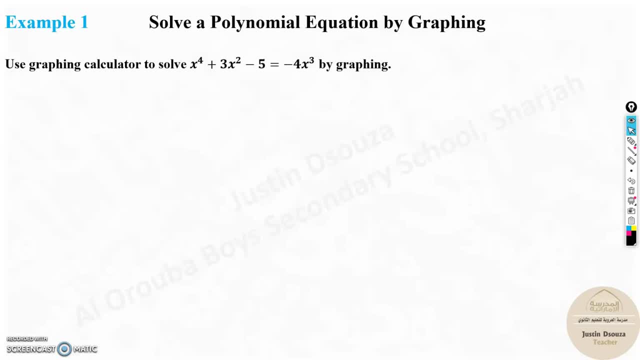 But we did not use graphing calculator, so it is fine. I'm not sure whether they'll be asking this in exam, but even if they ask and you have options given to you, you can find it directly by trial and error method. 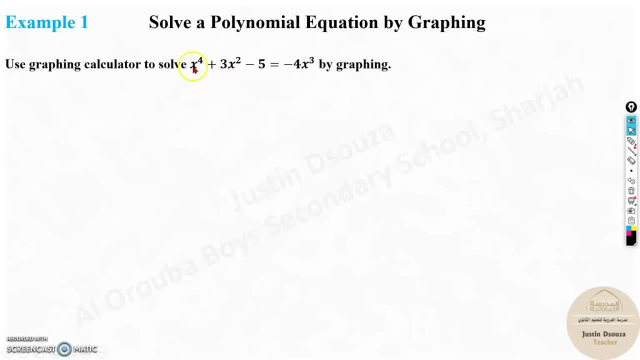 Now I'll tell you how is this solved. See now, the problem is it's x to the power 4.. Since it's x to the power 4, you can't solve it in your regular calculator. You need a graphing calculator. 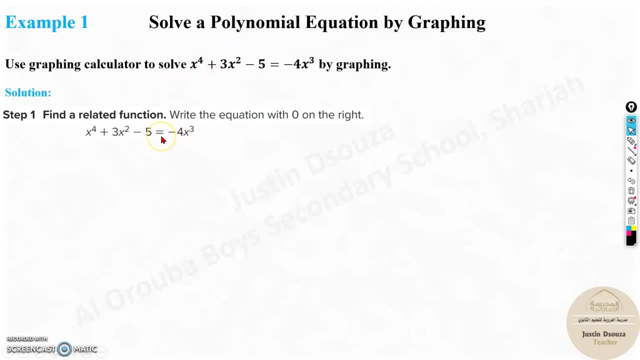 And the normal method is very onerous. It will be very tiring, It will take a long time. Now Here, find a related function. Related function means get everything to one side and make one side equals to 0. So over here you're adding minus 4x cubed. 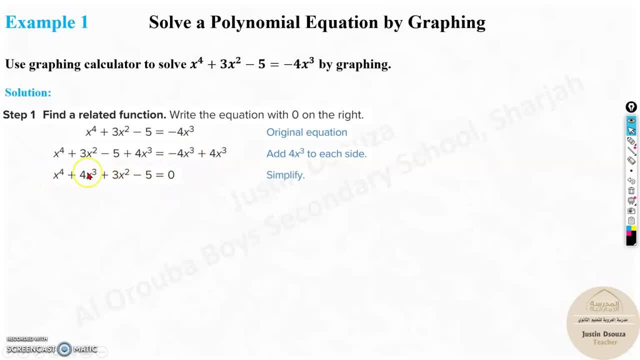 So this side will be 0 over here, And this is the thing. The related function is this function over here. Okay Now, if you want to find the solution, you should just solve this, making it equal to 0.. But how do you graph it? 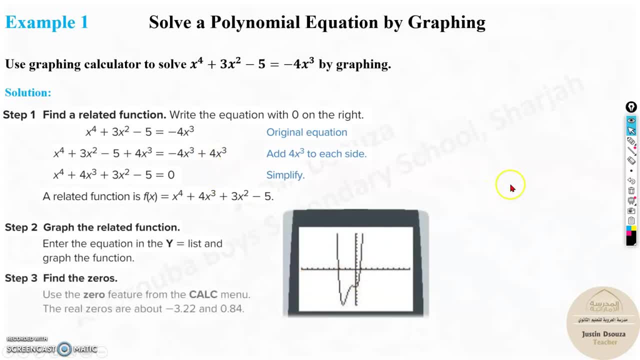 Now over here they have used graphing calculator. Now this is the graph over here. How would you? graph is basically taking values, Say the value of x as 0, as 1, 2, minus 1, minus 2.. Put it over here and then graph the points. 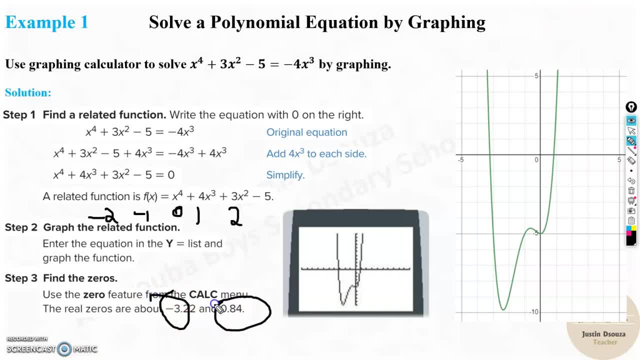 But even if you graph, it's very, very hard and difficult to find these x values. Okay, So you can take the approximate x values, But now, if it's just graphing and you've got four graphs, there's a trial and error method. 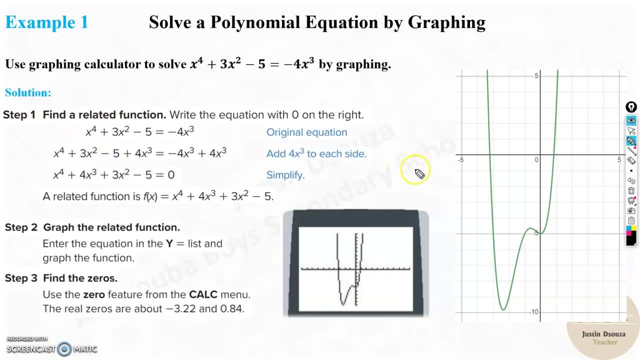 Now what this is. it's very simple. You will have four graphs with you. Choose any x value. I will start from 0.. Okay, I'll choose this x value as 0.. So, instead of this x in this given equation, the related equation put 0 instead of x. 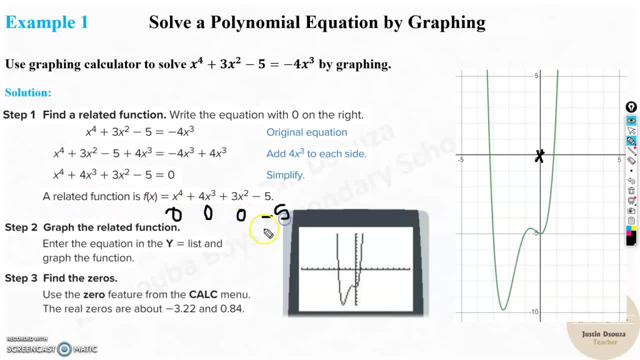 Everywhere this becomes 0.. What is remaining Minus 5 is what's remaining. So the answer over here would be minus 5.. Is it so? Yes, that is minus 5.. So that is the answer. That's it. 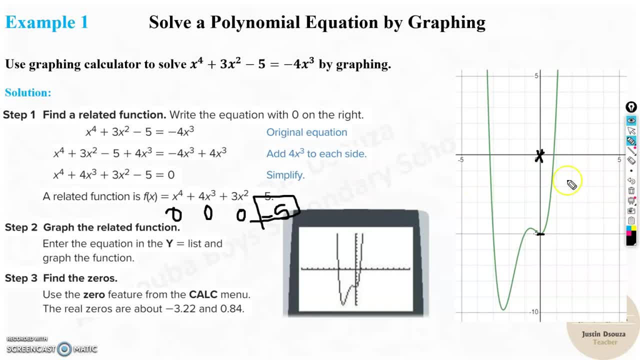 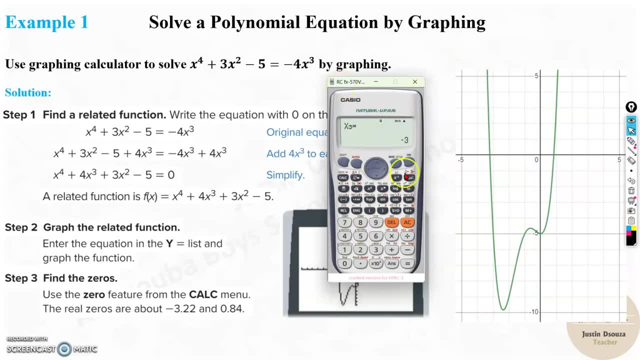 Now I'm sure there will be many answers with the same, you know: minus 5.. So how about we change it? Let's say, take negative 2 over here. So you will have to. let's go back over here. Now what you will have to do is, instead of x, you need to put minus 2.. 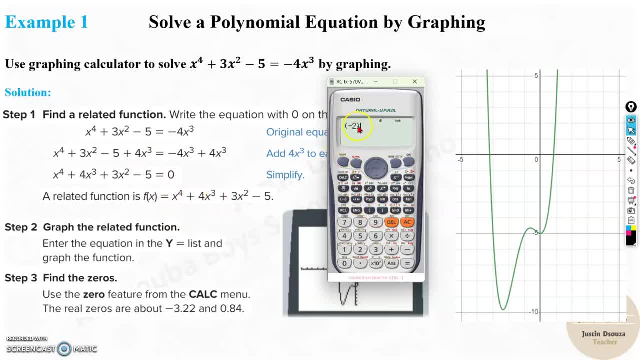 Please remember, use brackets when it is negative numbers, so you will get the exact answer. I'll show you why. Because if it's an even power, If it's a 4, the answer over here is 16.. Right, But let me make it an odd power. 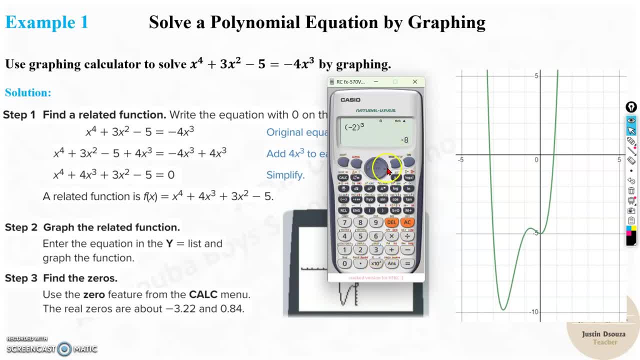 That will be minus 8.. So it makes a lot of difference. And now say, for example: if I don't use the bracket, Okay, I'm deviating, but let it be because I want you to know. See, if the minus sign is within the bracket over here, you will get positive 4.. 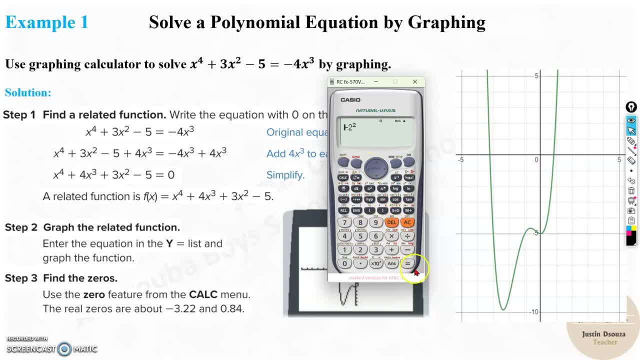 Right Now I'll remove the bracket And I'll show you The same thing. It is negative 4.. The answer is not same, So that is why, whenever you see negative numbers, it's most crucial that you put the brackets. 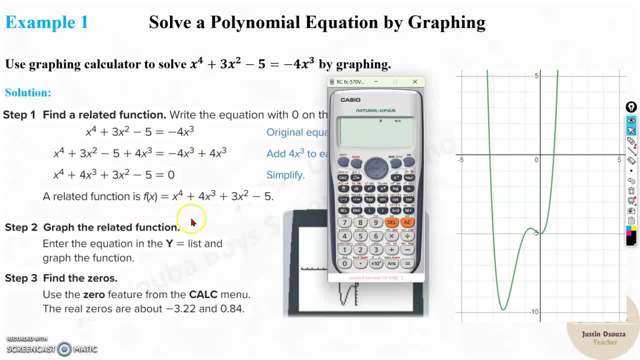 Now I will, I'll assume I'll try to find the value of minus 2.. Let me put over here, instead of x, as minus 2 inside the brackets, and power 4. Plus 4 times x is again minus 2.. 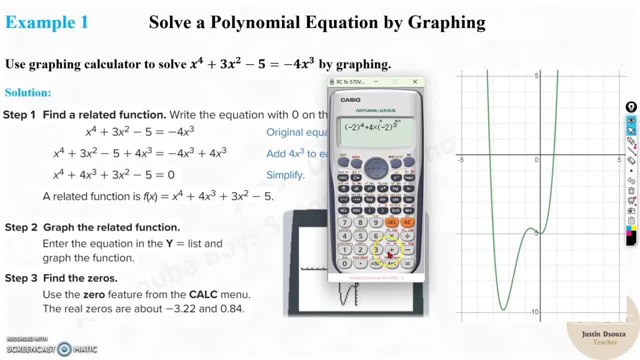 Close the bracket and x to the power 3.. Lastly, we have plus 3 into minus 2, the whole square, 2, the whole square And negative 5.. The answer is minus 9.. And look over here Let's compare. 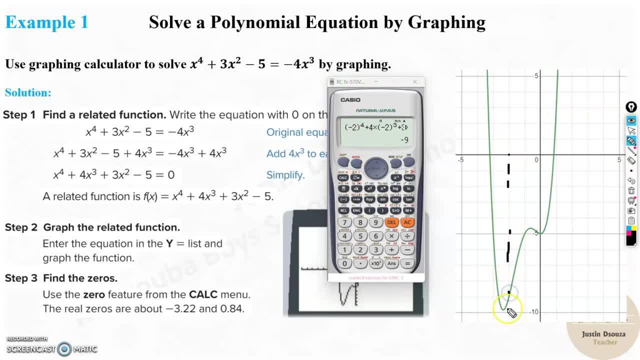 This is 2.. See, this is the value of 2.. Now, if you look closely, yes, it's about 9.. Okay, Now I can't zoom over here, but still it's corresponding to 9.. It should correspond to 9.. 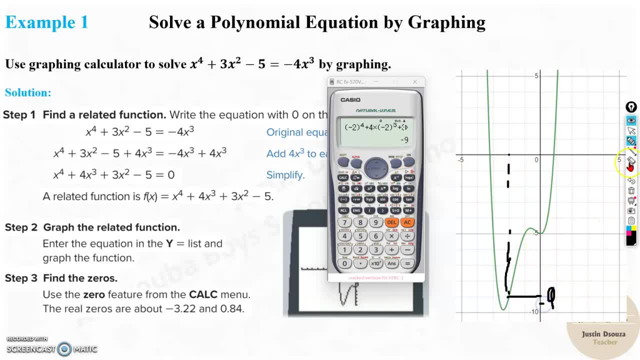 So that is the answer. It's minus 9 in the downside. So this is how you can directly get the answer of the graphs. Now, what you must do is the trial error method. Now what if, even at minus 9, there are two graphs? 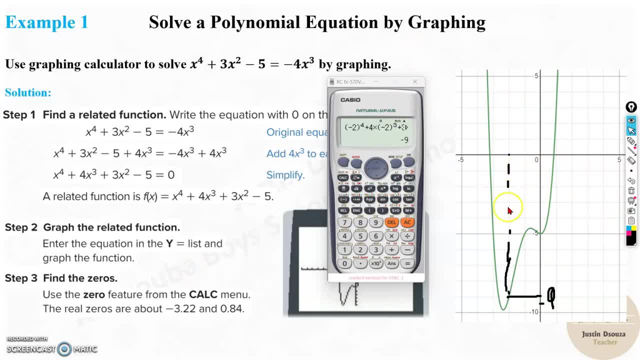 The two will be eliminated, but two are remaining. Try one more point. There will be only one graph for one particular function, So you can easily find the correct answer by trial and error. I hope this is clear. So this is how we can try.